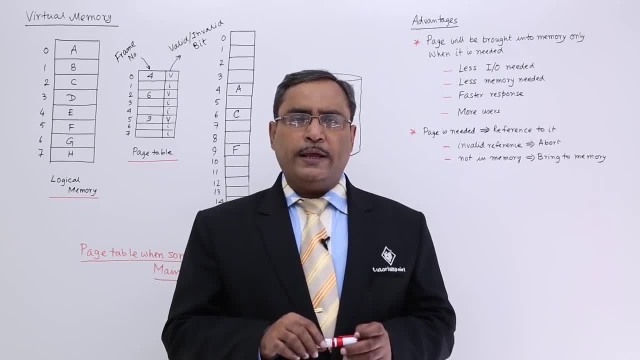 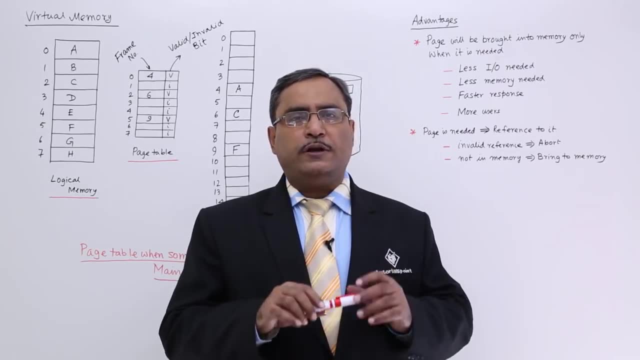 people, users are pressing F1. So there is no need to bring or brought or load the help module onto the computer's memory when the program has been initiated for execution. So the basic theme in virtual memory is that we shall load a certain piece of software in the computer's memory. 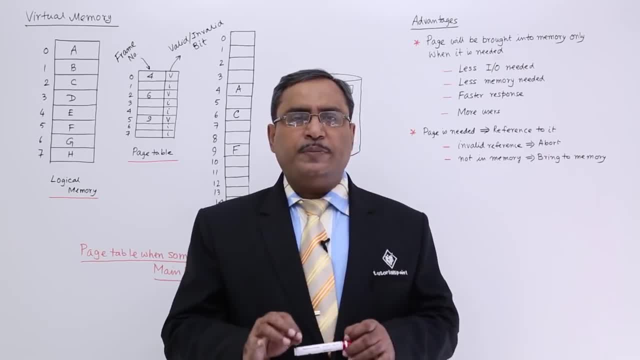 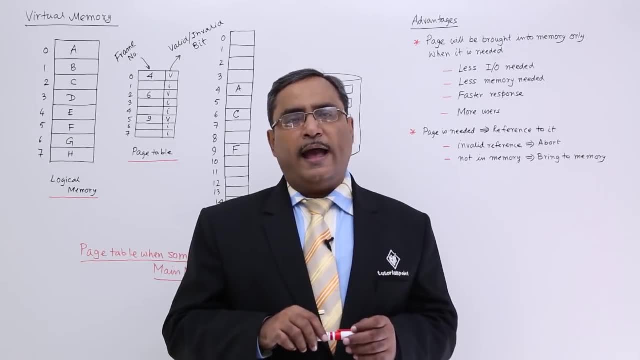 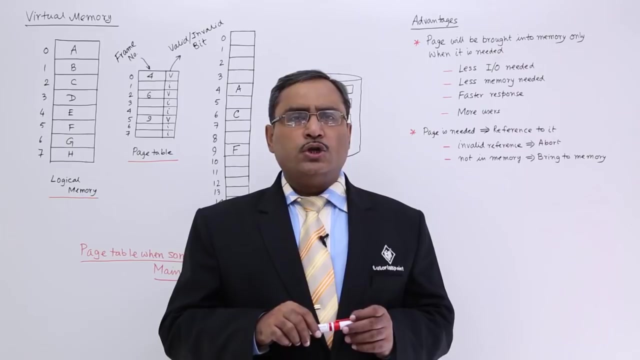 page onto the computer's frame whenever it has been asked for. So as a result of that, we shall we shall enjoy multifold advantages, As we are loading fewer number of pages, as when required, onto the computer's memory. So the effective loading time of the program. 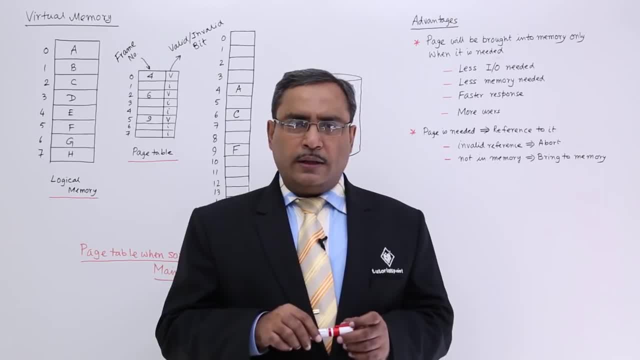 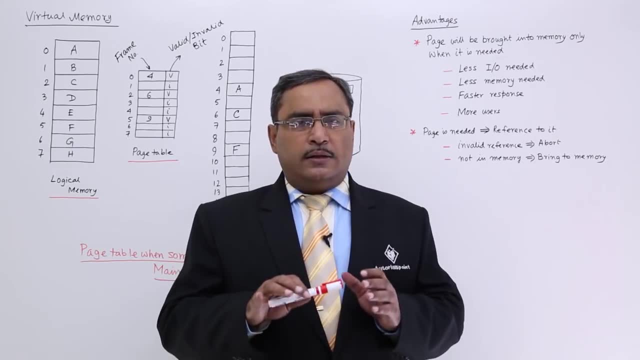 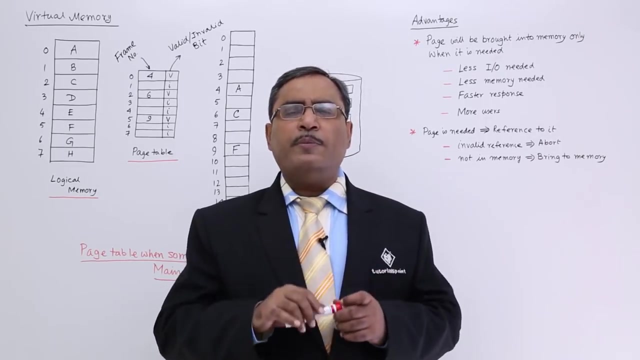 will be minimum and user will feel that he is having, or she is having, a very smooth execution of the program. So he or she will feel that he or she is working in a huge memory space, but that is not true. He or she is working a very limited amount of memory space in the 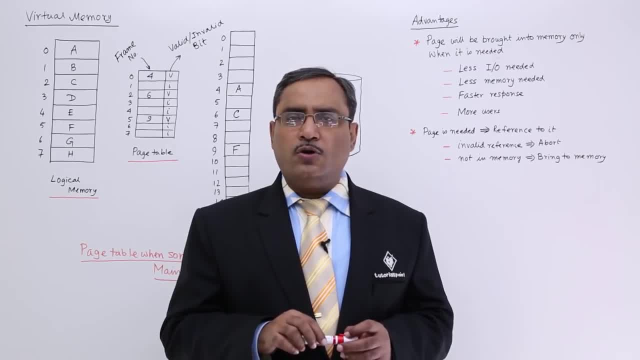 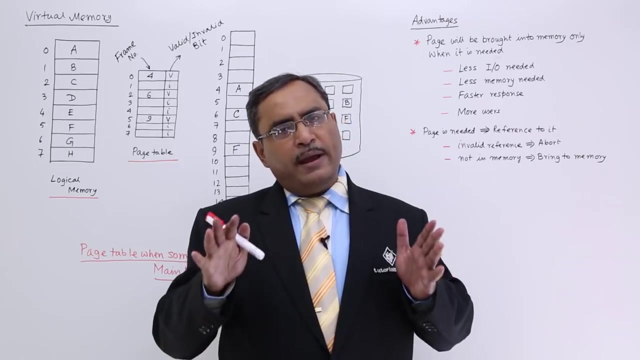 computer's memory because the full program has got not loaded initially, And also for each and every program if we have a partial memory space allocation, So at a time I can load multiple programs in the computer's memory using the same main memory space. 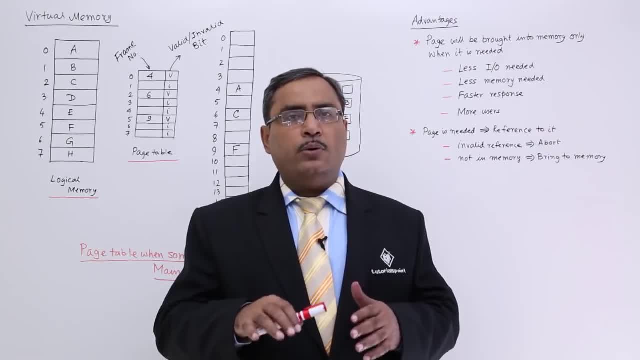 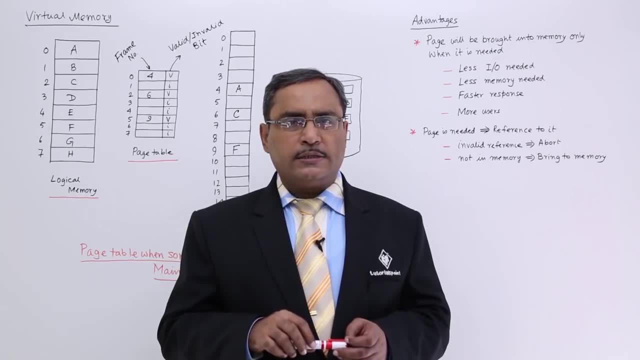 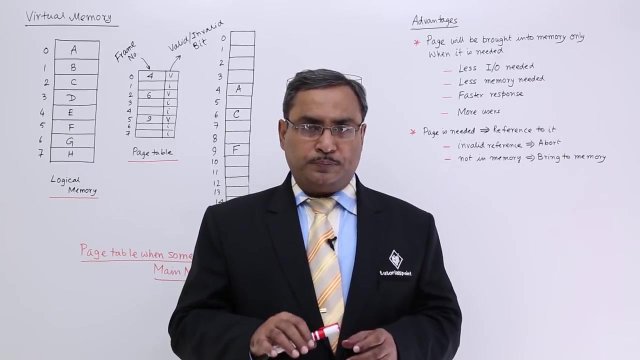 So what will happen? The degree of multiprogramming will increase. The degree of multiprogramming means the number of programs that can be executed simultaneously inside the computer, inside the computer's memory. So that is the main advantages. So to describe this particular, 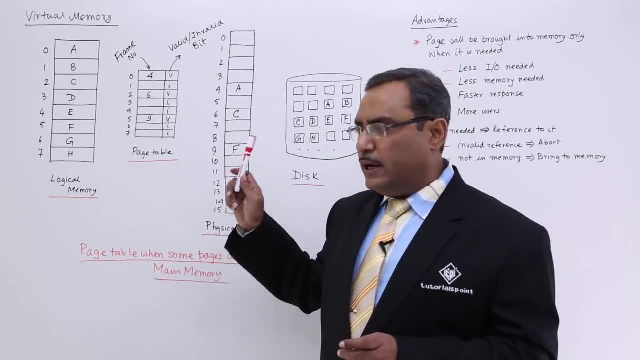 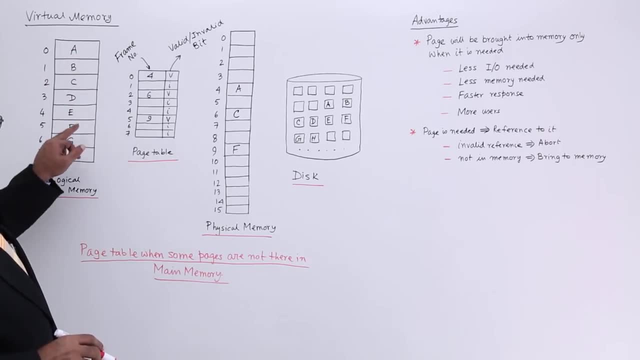 concept we have. we are having one diagram here, So let me discuss this diagram, then I shall go for the text. So now here you see, here we are having one program. This is the program which is in the logical memory. How many pages are you? 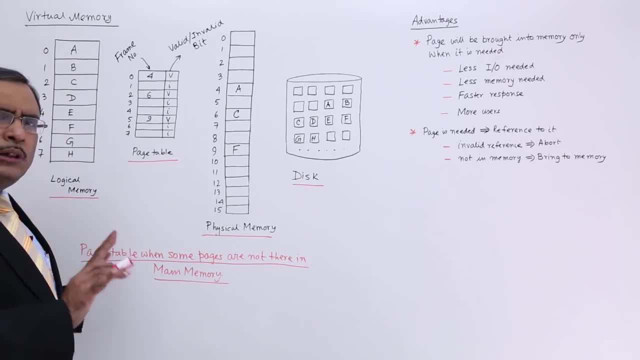 having here? We are having 7 pages. Let us suppose all the 7 pages are there to hold this particular program's content. So 7 pages are there. to mark them. I have written a to h. Ok, all these 7 pages, rather 8 pages, because 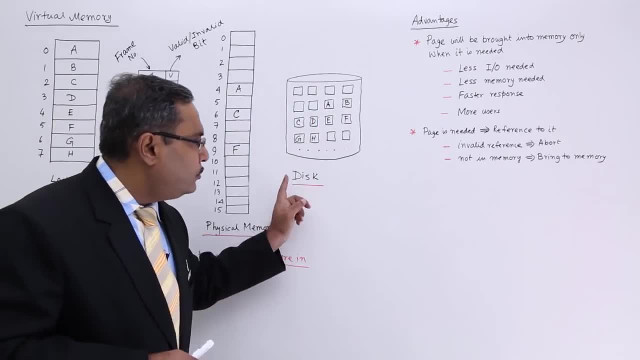 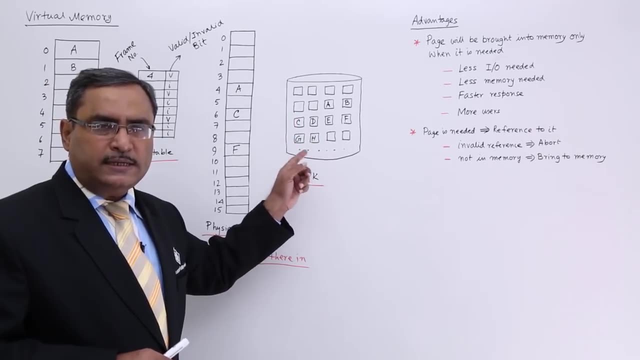 it is starting from 0.. All these 8 pages are now residing on to the disk, All these 8 pages deciding in the disk: a, b, c, d. in this way, if you proceed, you are getting all the 8 pages available on the disk. so in the physical storage, in the physical memory, full program is existing. 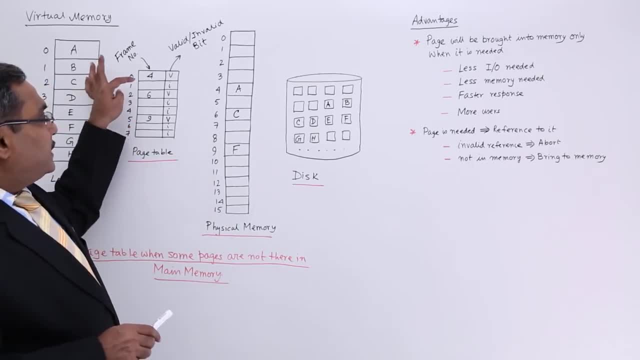 so that is no issues. but you see so out of this pages, this page number 4, that means that is e, that is e. page number 4 is e, so e has got loaded. page number 4 has got loaded. i am not loading e, i am loading a. ok, now see page number 0. that is a. i am marking this. 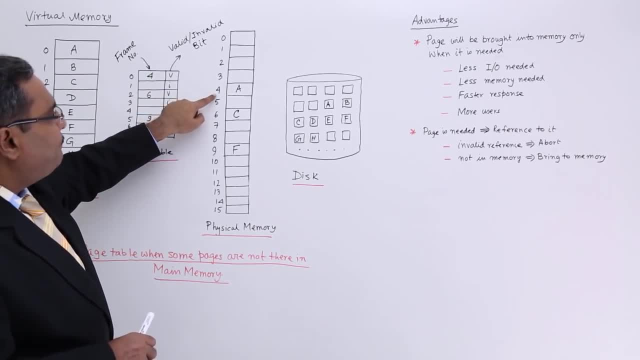 one, that it has got loaded in the frame number 4 going for another one. so i am going for c. ok, so page number 2 is c. so you see, in this particular page map table if you come to this second location then you are getting 6. that means the page c has got loaded on to the 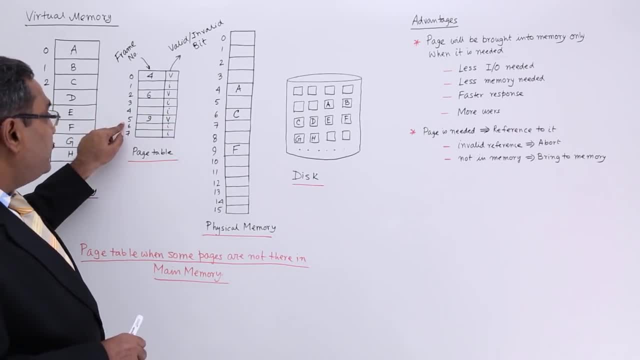 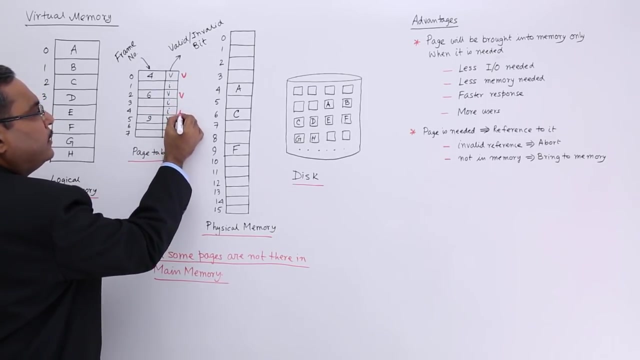 sixth frame. ok, and in this way the page number 5, which is f, has got loaded on to the ninth frame. that means, out of this 8 pages, i have loaded only three of them, so the respectively i am writing here, valid, valid, valid. so this three are the valid and rest are invalids. why? because they 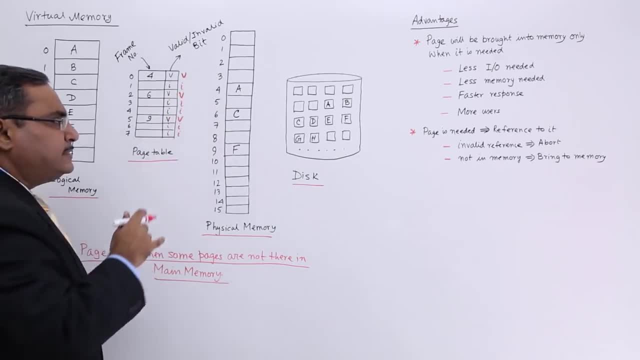 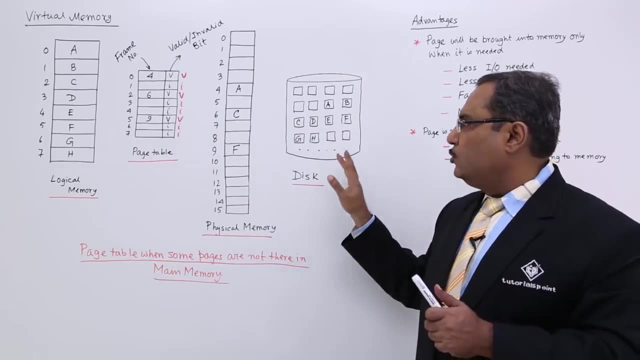 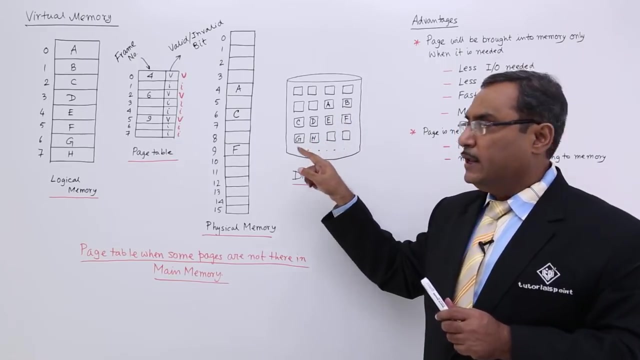 have not got loaded on to the computers memory at this instant of time, so let me explain the diagram again. all the pages are existing on to the physical storage. that is my hard disc. it is there a to h, everyone is there. these are logical address space where having 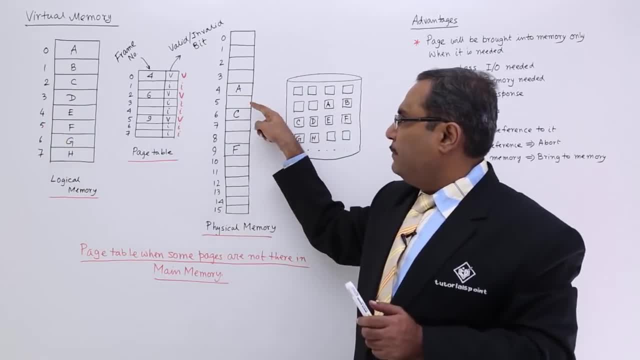 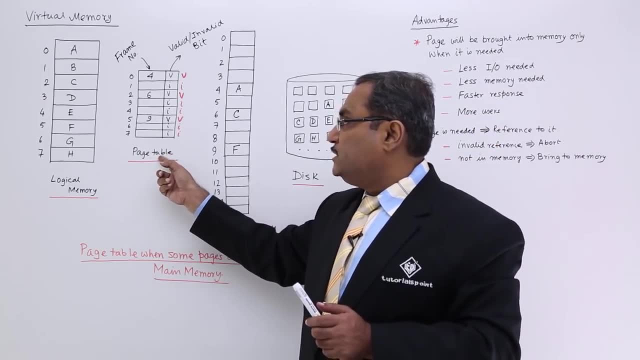 8 such pages. out of them, only three of them have got loaded. so this page has got loaded, to which frame? that is the purpose of the page map table: to hold the information. so page 0 is a. page 0 has gotten loaded on to the physical storage that is my hard disk. it is, it is there. 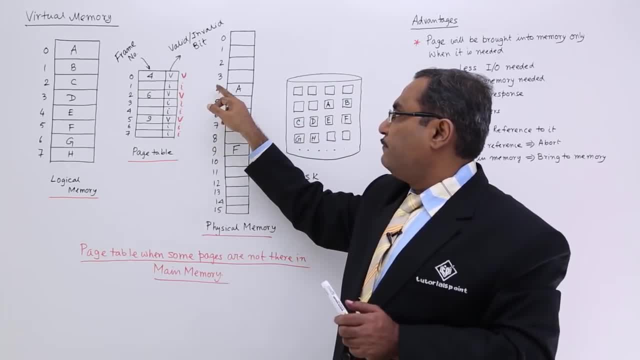 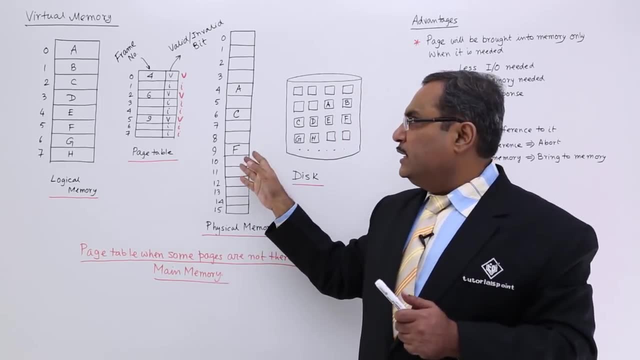 a to jh. every one is there. this are logical address space where having eight such pages to the fourth frame. if you come to fourth frame, you are getting a. similarly for c and f. so what has happened, you see, initially, only three pages have got loaded onto the main. 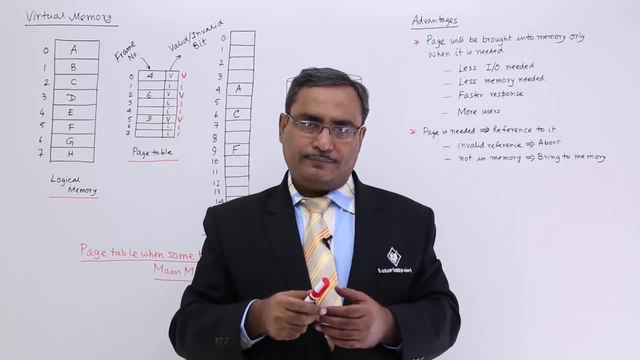 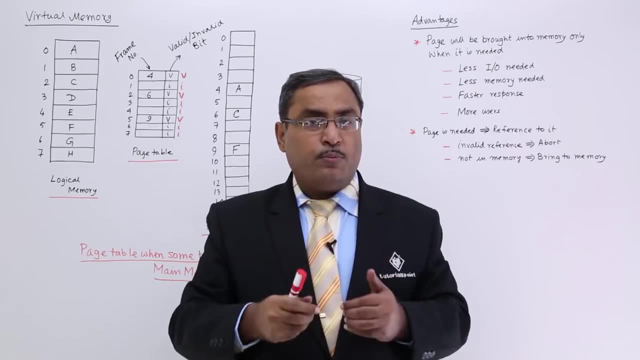 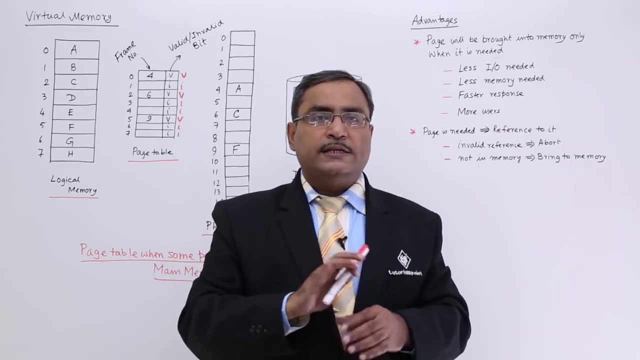 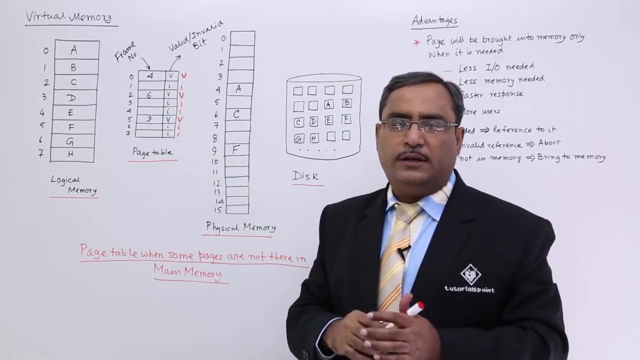 memory. so the program will be in execution. whenever a particular page has been called and the page is not there existing in the main memory, then the page has to be brought and bringing this particular page to a new frame is no issue. but if this particular process is having only three frames for its allocation, then in the case to make the fourth page available, 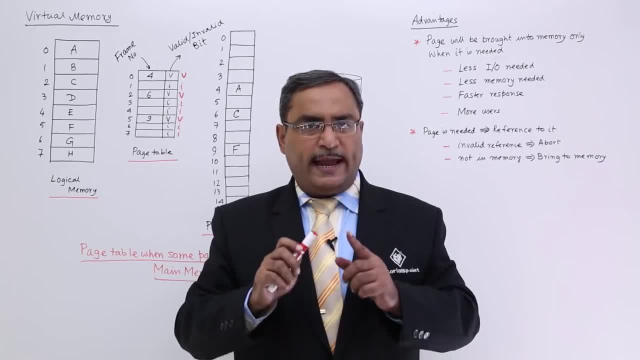 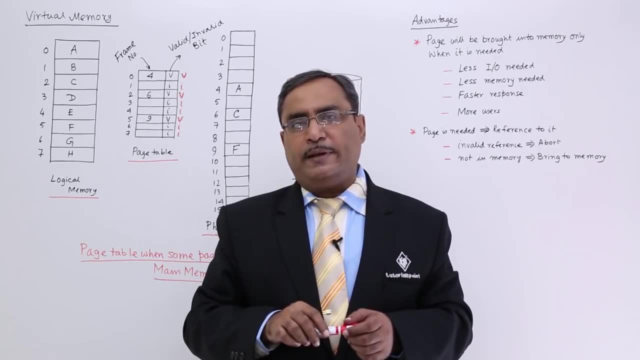 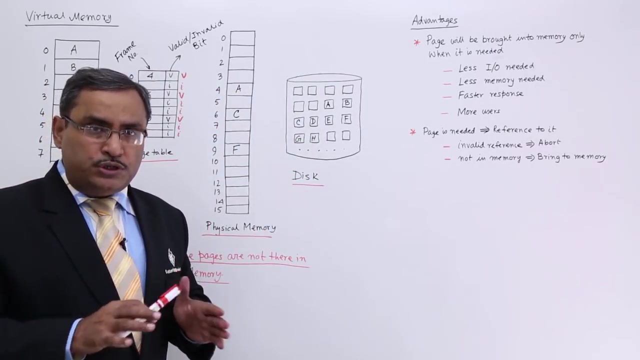 there i must be replacing one of the previously existing pages from this particular main memory, so algorithms will be coming, known as the page replacement algorithms, that will be coming in the next videos and that is the concept and user will have a very smooth journey. user will have a very smooth execution of this. 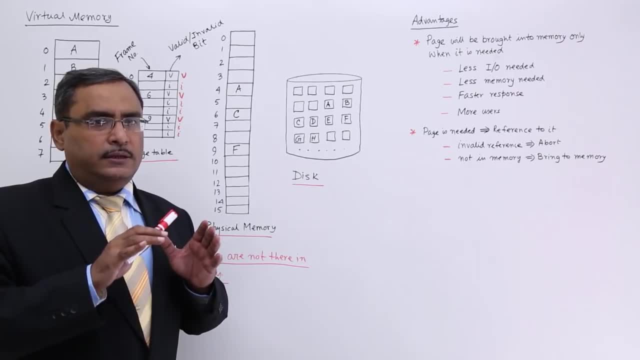 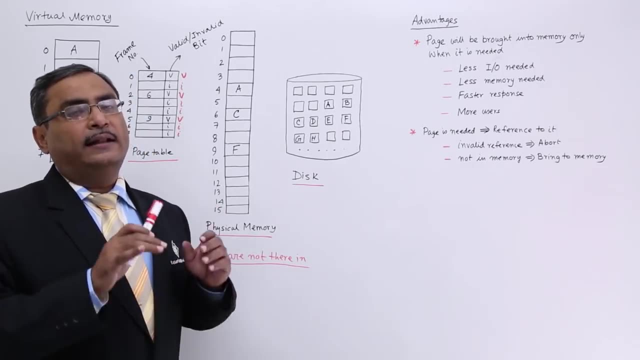 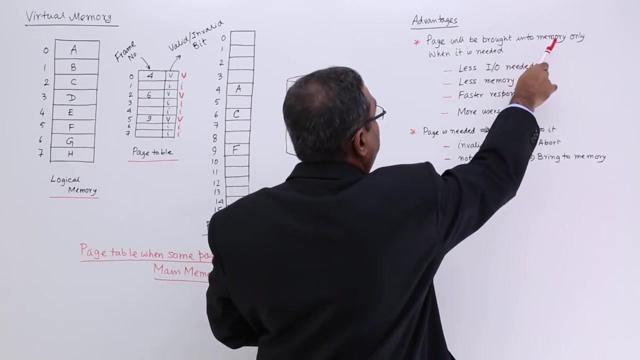 program. so he or she will feel that the program is working in a huge space, but that is not true. the program is working in a very limited amount of space and that is why it is called virtual memory. see what are the advantages. page will be brought into the memory only. 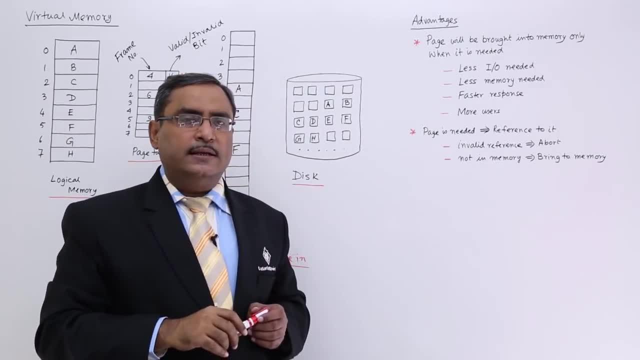 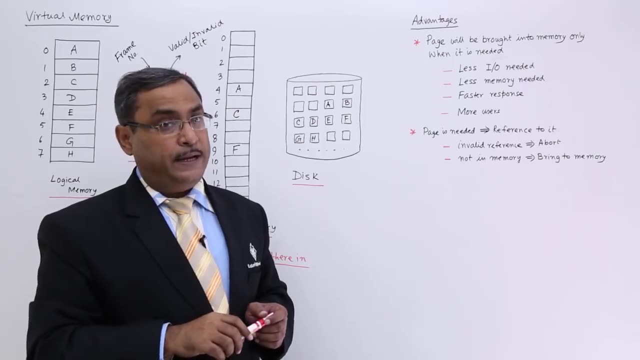 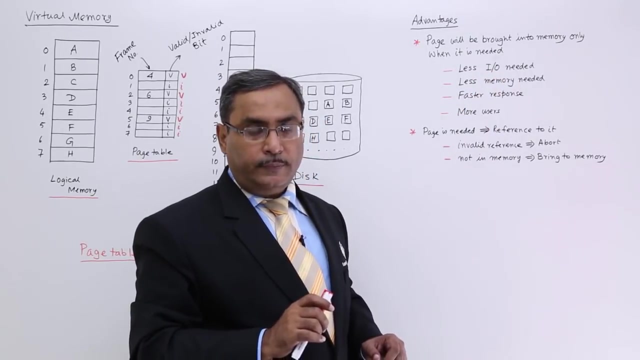 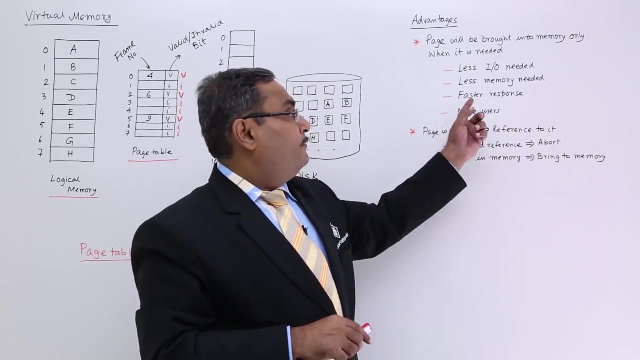 when it is needed. this is known as lazy swapping. lazy swapping: let it be demanded, then it will be loaded, and also it is known as demand paging. so what will happen? you are not loading the full program, so let i o required. you are not loading the full program into the computers. memory: less memory needed. faster response. 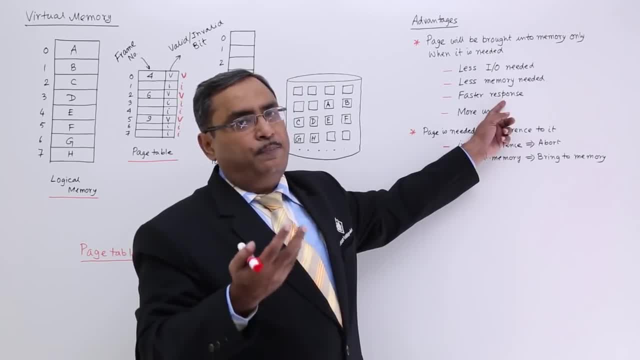 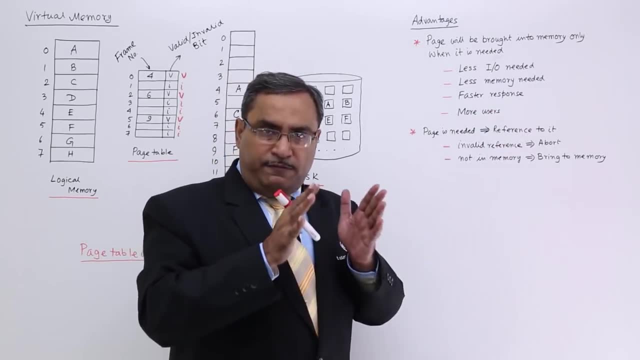 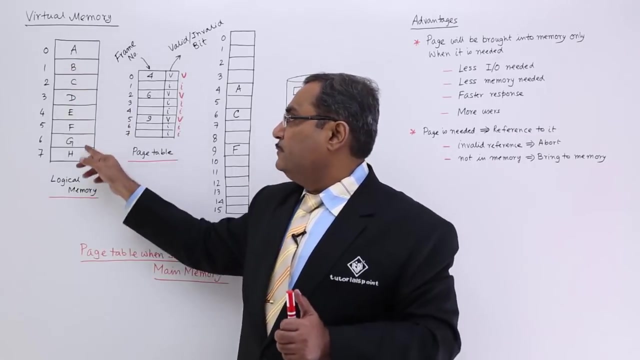 as the loading time is lesser. so what will happen? the program execution can initiate after loading required number of pages into the main memory. and more users, because if part program, part process, if we require fewer number of frames out of eight frames, i require only three of them. so the rest of the frames which are available, in the physical memory can be used for loading other programs of other users, so more users can access the same memory. so also you can increase the degree of multi programming. degree of multi programming means the number of programs that can be loaded into the main memory and the number of programs that can be loaded into the main memory and the number of programs. 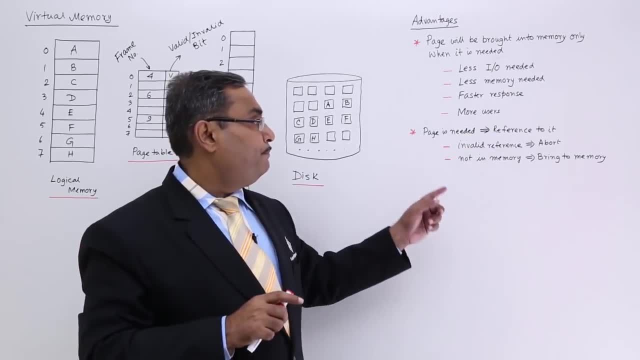 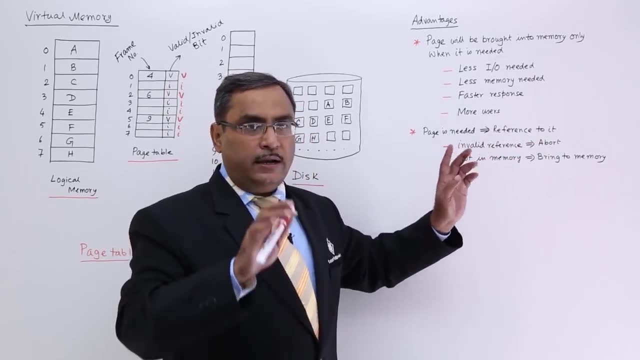 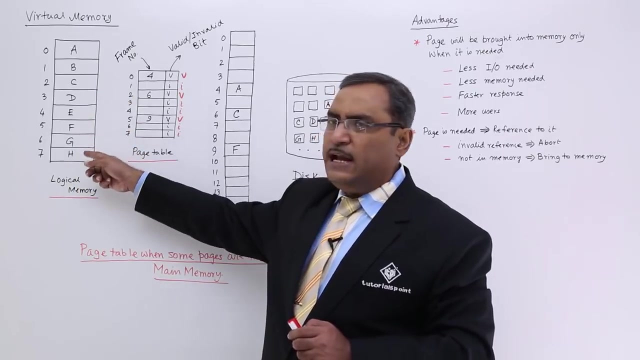 executing at the same time in the computer's memory. so page is needed, then it will be referenced if the reference is invalid. let us suppose i want to load the tenth page of this particular program. you see, tenth page is not there. we are having only eight pages, so that tenth